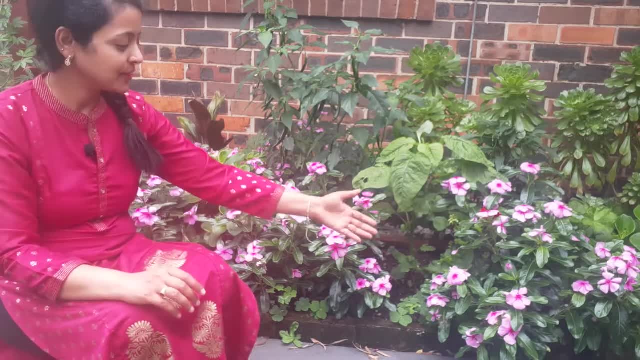 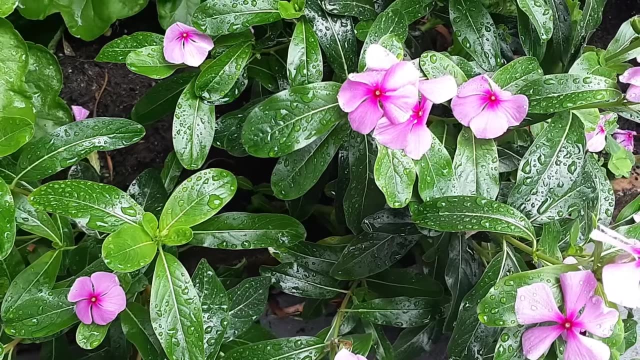 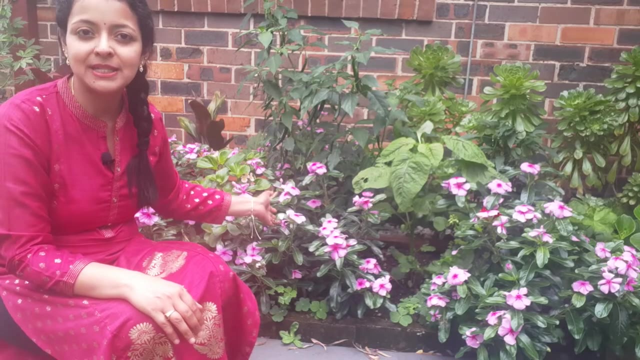 So, friends, today we will be talking about this beautiful plant that you can see in front of you. This plant is known as Vinca periwinkle or Vinca flower, And I'm pretty sure most of us would be familiar with this plant because it is very popular and can be seen grown in your front yard or backyard. 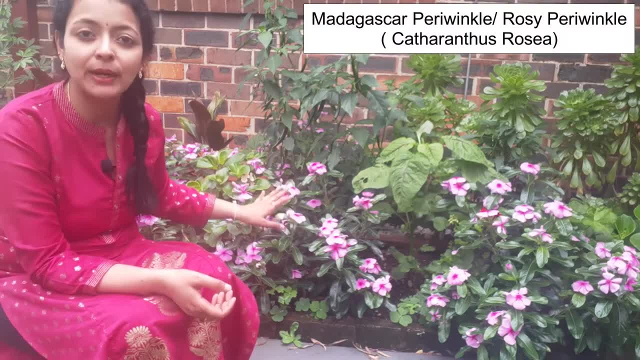 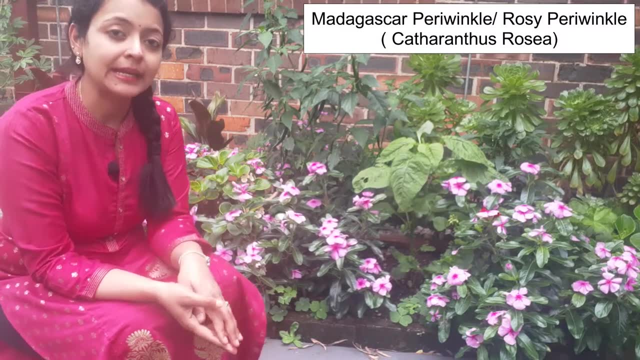 Now, this plant is also known as Madagascar periwinkle, And why? Because it belongs, it is native- to the Madagascar. This plant is a type of plant grown in southern Europe and India. In India, it is also known as dieser bhowar. 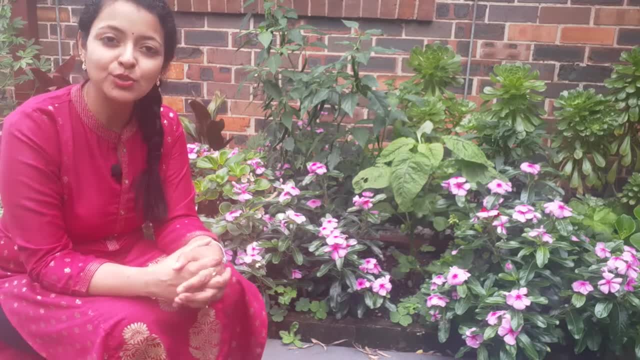 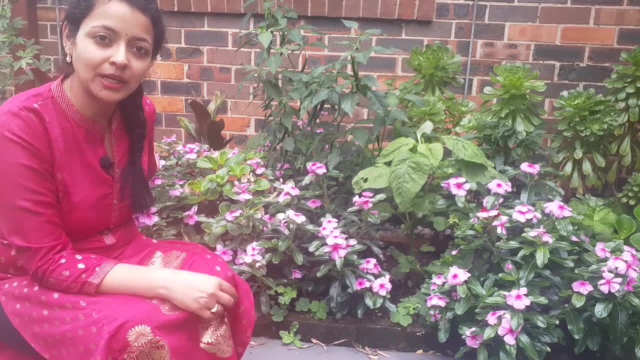 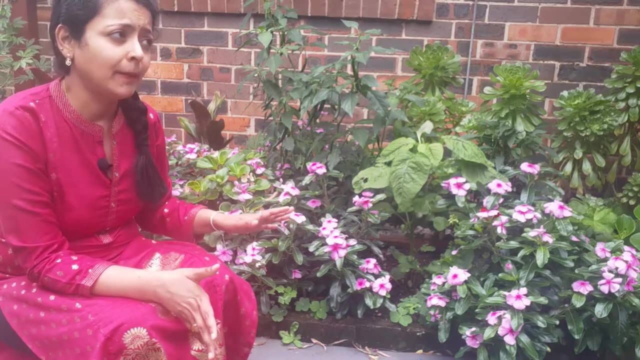 Besides being a Golden blooming plant, it isİis always blooming In the early spring of this year in Australia, which was September. This time it is January, which is in mid-summer, And look at this beautiful flower. It is quite hot. 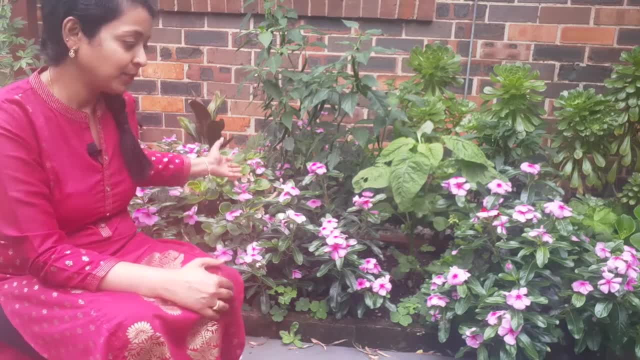 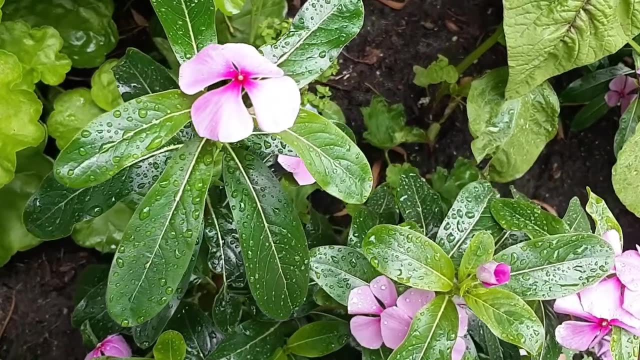 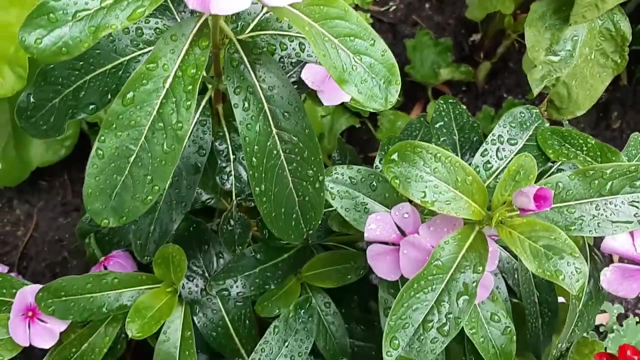 because it is degree temperature and but look at the bloom: it's so nice, so healthy, so lively, so that's that's type of temperature that they like. so they would start blooming in the spring season until late summer and and the warm temperature and the warm, humid climate is what they love. these plants are drought tolerant plants. as well. so even if you don't water, or even in those areas where normal grass does not grow like rocky surfaces, these plants can grow and survive very well, but over watering can definitely kill these plants. these plants can also withstand the sunny spot, so if you want to grow them in a sunny area, that is. 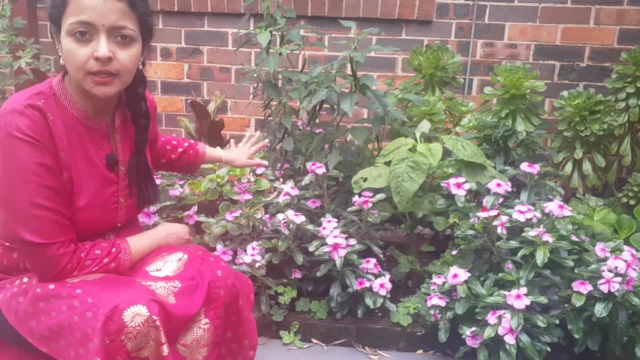 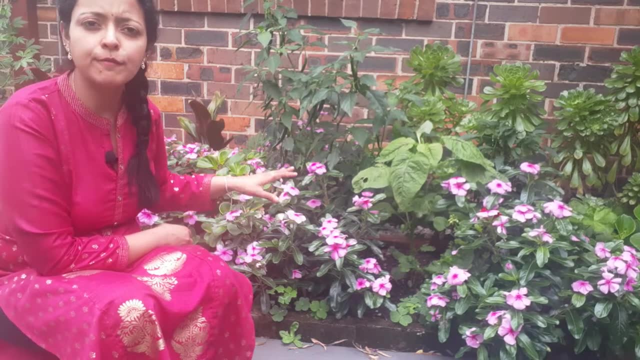 also fine. so this area of my garden usually receives shade- partly shade- throughout the day, so around 5 o'clock I can say, or 435 o'clock during summer season. so that's what I like to do in the summer. so that's what I like to do. 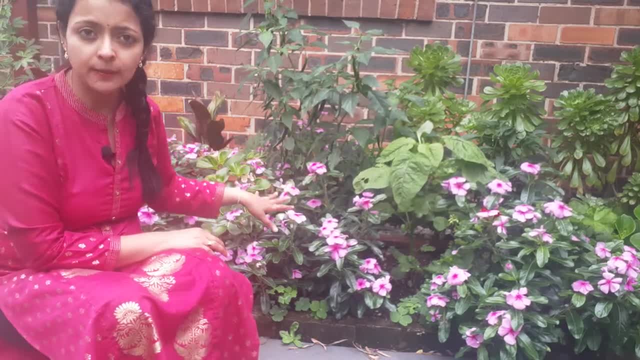 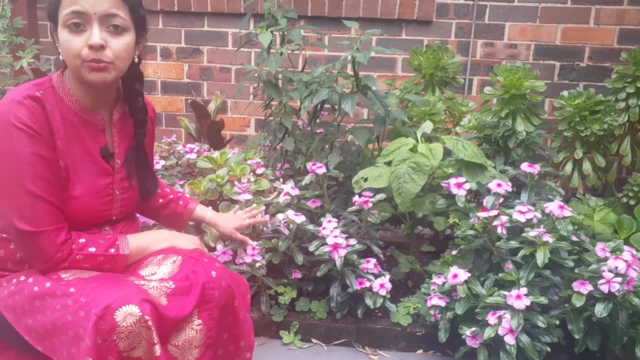 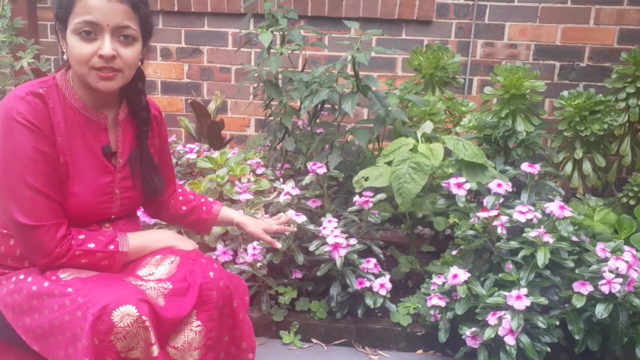 season this part of the garden gets the full Sun, but that Sun is not very harsh, so in that part shade this plant is doing really well. you can make out with the beautiful leaves and the flowers flower display that these plants are doing really great. so part shade is the one which is preferred for these plants. 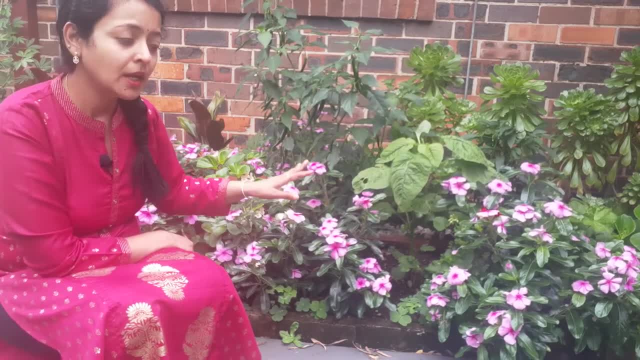 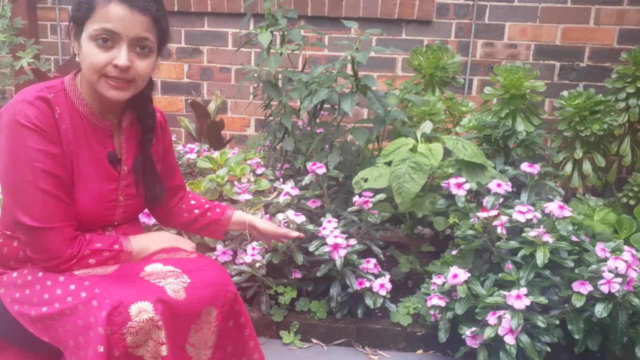 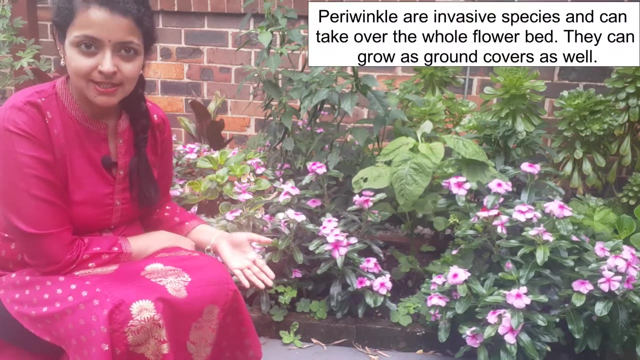 but if you want to grow them in full Sun, that's also okay for these plants. these plants prefer to be grown directly in the ground and they can grow as a feed. honestly, all these plants that you can see in front of you, none of them I have planted in this season. none of them I don't know. 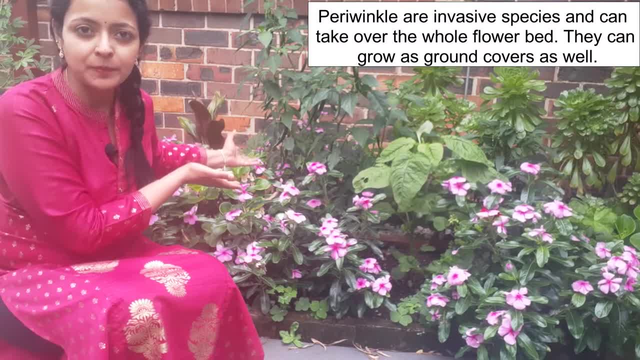 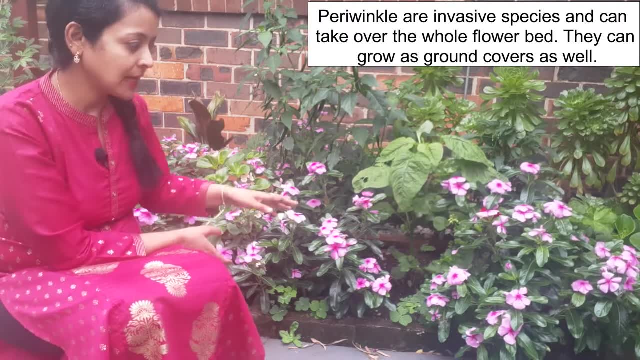 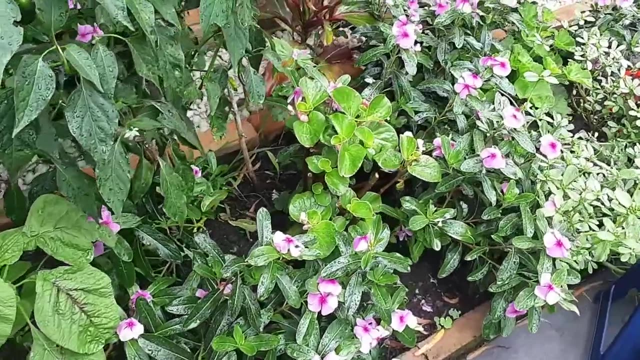 from out of where all these plants just came up in spring and since then they are blooming beautifully. I haven't grown any single one of them and they grow like a weed. as you can see, it has covered my whole garden bed and it grows like a weed. they're very, very difficult to remove or very, very. 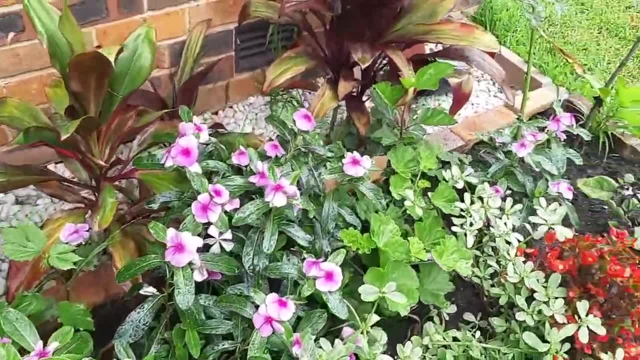 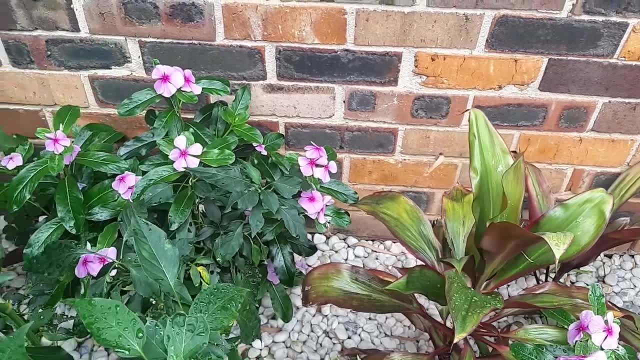 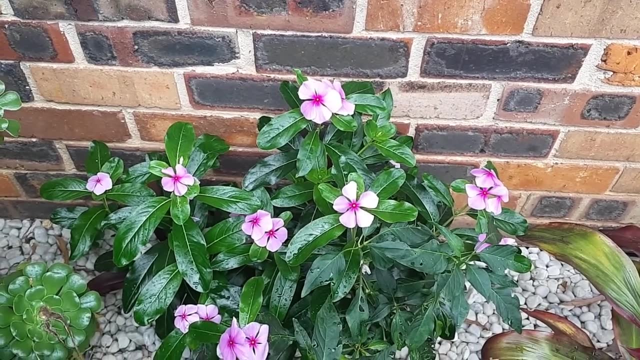 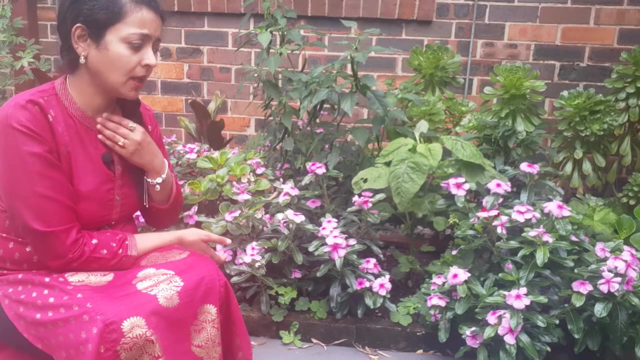 difficult to kill, but they look very beautiful. they help to reduce this problem of soil erosion because of the ability to grow anywhere, and they hardly need any maintenance. to be honest, other than the rainwater or the water that I give in my garden, I have never fertilized them, never done anything special for them, and they are 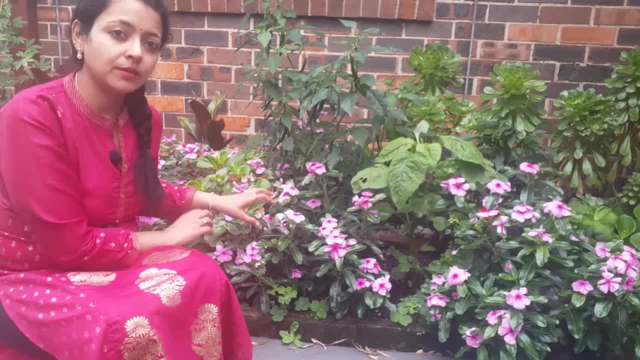 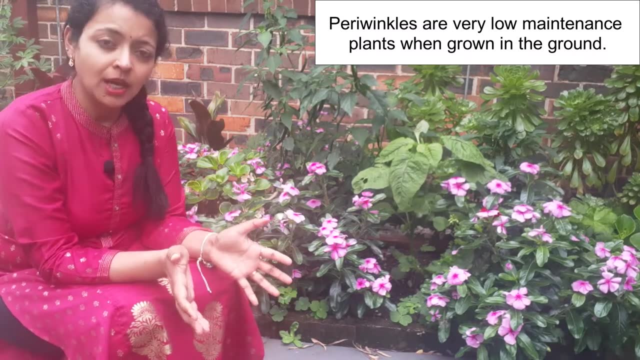 doing just great. so if you are growing them in the ground, there is very much low maintenance. you don't need to maintain them at all. but if you're growing them in a pot, make sure that you use well draining soil and make sure you add perlite or 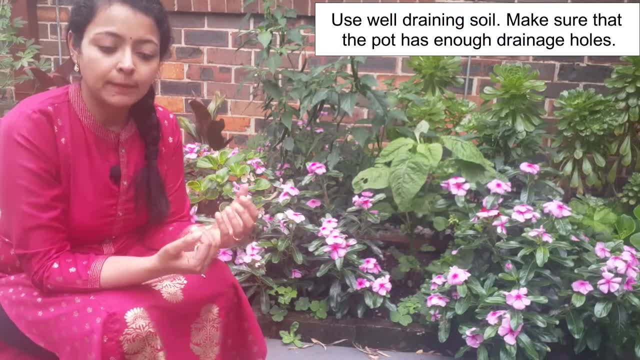 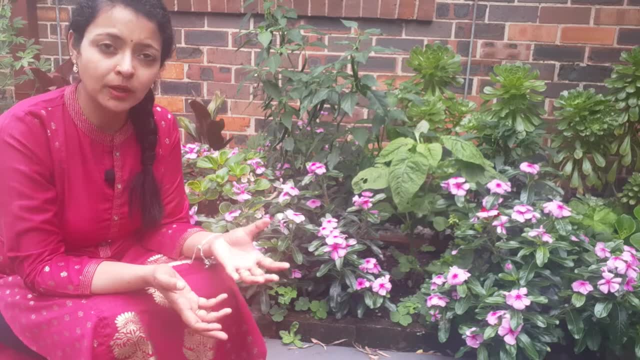 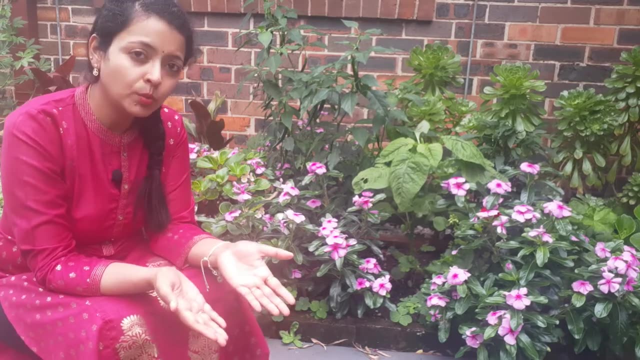 coarse sand or some sort of material, pumice, some sort of material which can allow better drainage, so that the plant is not sitting in the soggy soil, because that is the only thing that can kill these plants, and make sure your pot has got enough of drain, each holds. if you want, you can fertilize these plants. 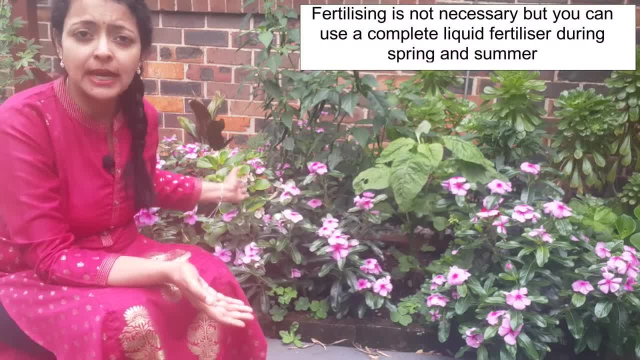 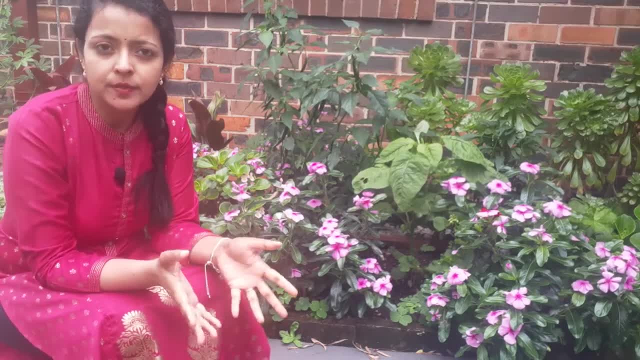 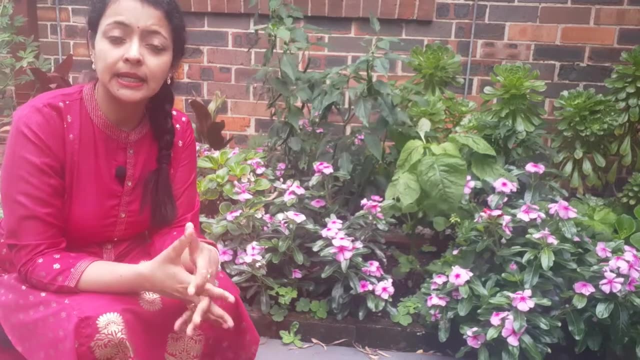 but I have not fertilized them throughout spring and summer and they are still doing very great. but if you want, you can use a complete liquid fertilizer of the dilution and fertilize your plants during spring and summer. then next is the lighting condition. as I said, they love partial shade temperature. 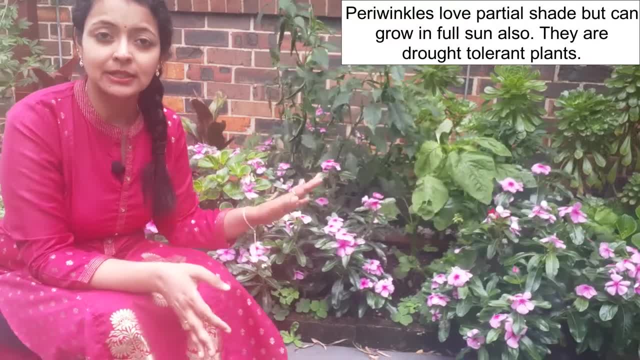 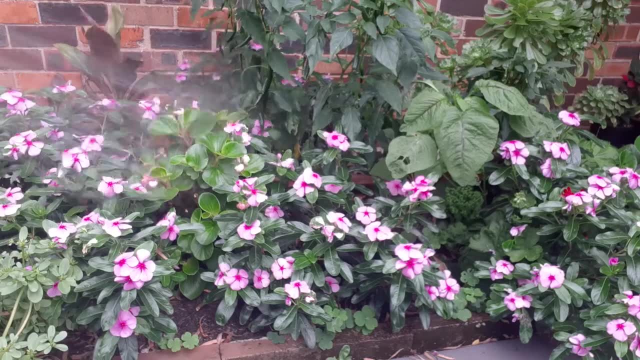 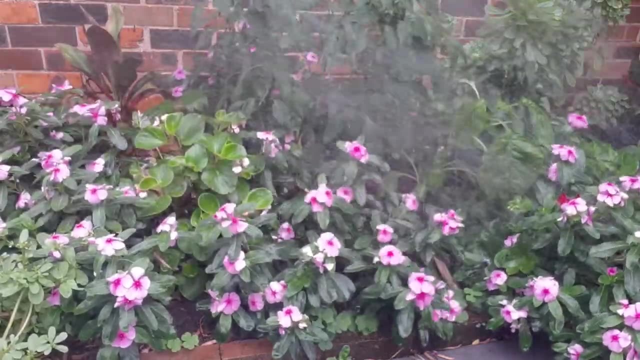 hot, humid and warm temperature is what these plants like. and watering when they are in the ground, you can water them every day, like I water all the whole my garden every single day. I water these plants every day. they are happy. they are healthy. the soil is always moist, but if you are growing them in a pot, always. 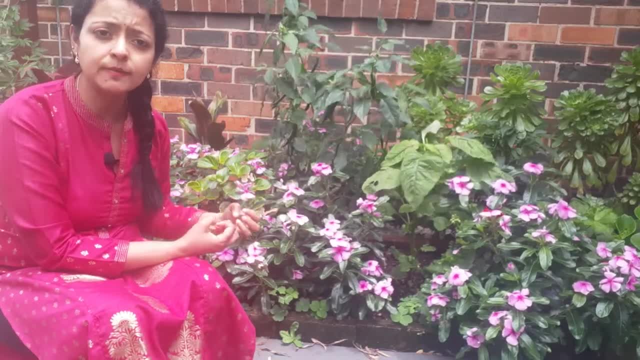 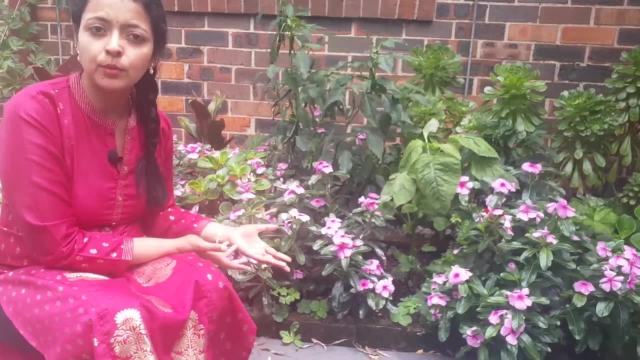 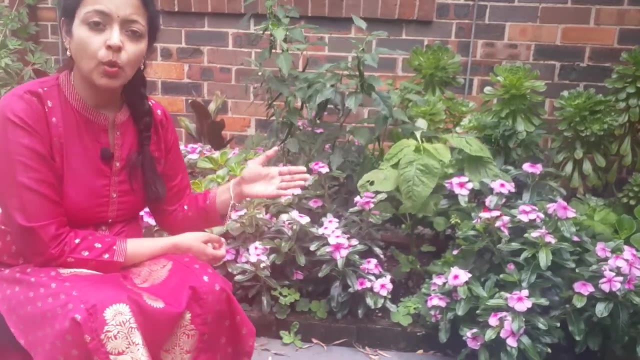 check the soil before you are watering. so if the soil is very wet and moist already, do not water it. leave for few more days and see how the soil- whether the soil has dried out or not- and the soil is dried up, water it then. so do not over water them because it can cause root rot and your plant. 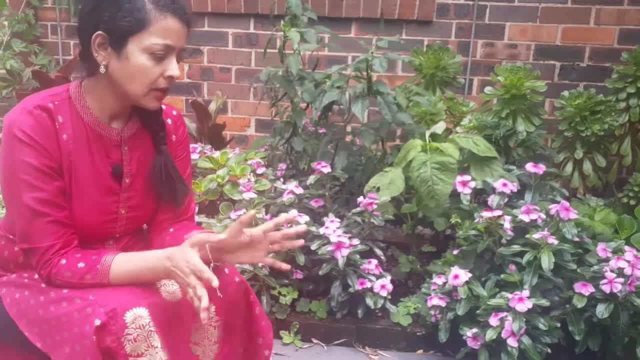 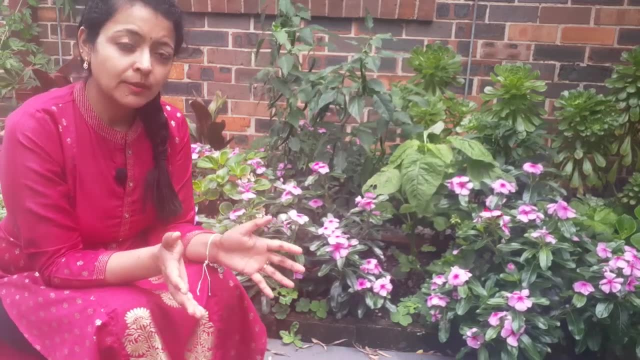 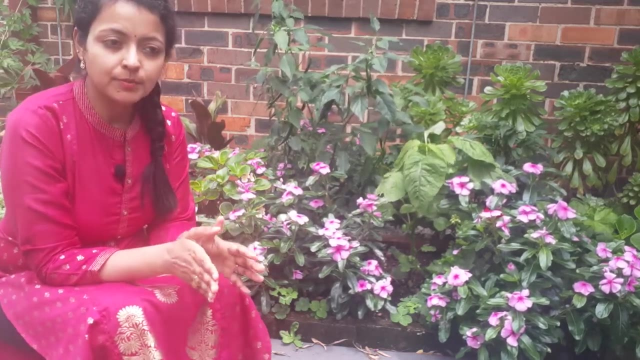 will die, so do not over water these plants. there are some problems, like if you are planting this plant in a pot, then you sometimes you might see the yellowing of the leaves or the leaves falling over and drooping. now, that happens most of the times when you are planting these plants in the pot, because 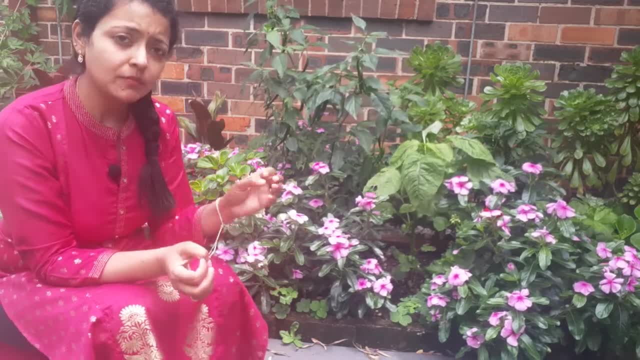 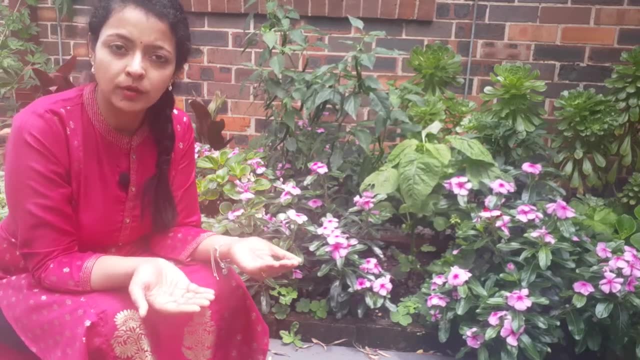 in the pot. if you are over watering your plant, the leaves will start turning yellow- the lower leaves or the upper leaves. it will start turning yellow and they will start falling over. and if you are facing the problem of yellowing of the leaves and then falling over, that means you. 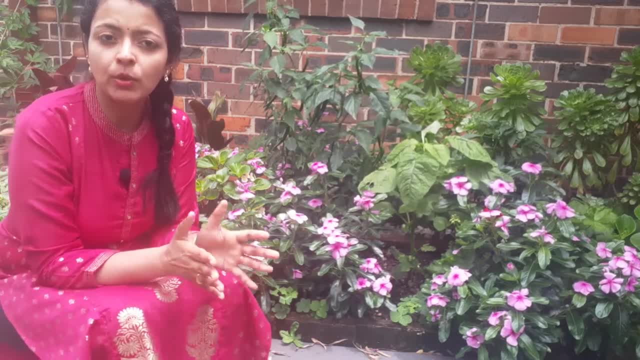 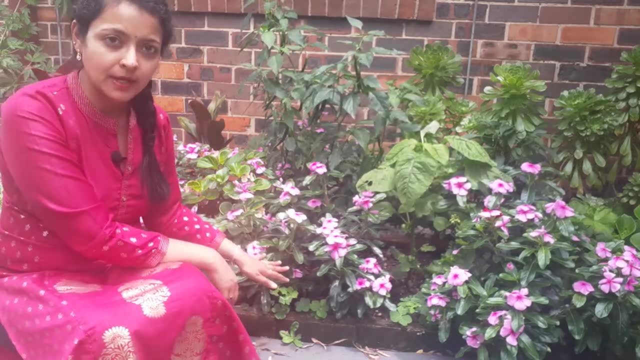 have under watered your plant. so this mostly arises when you are planting them in a pot. but if you are growing them in the soil itself, in the ground itself, this problem hardly arises. like these plants, I water them every day. look at the beautiful foliage of this plant. 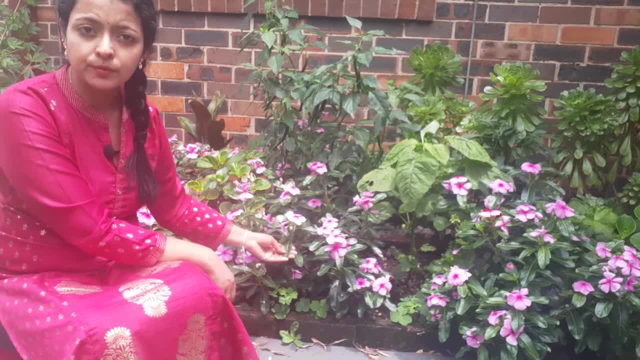 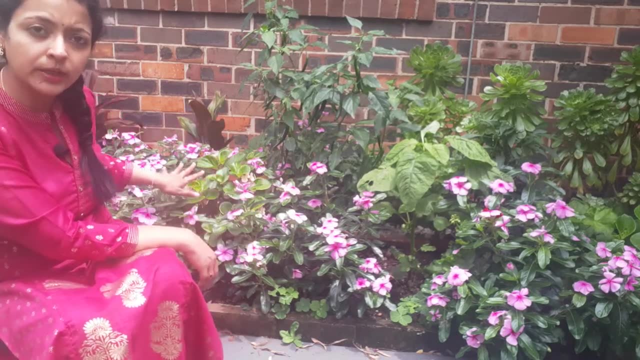 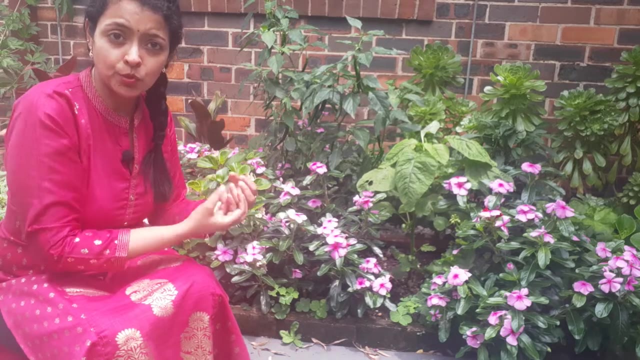 shiny and beautiful. shiny, vibrant, they are so beautiful. There is no yellow leaf in all these flowers, no yellow leaves, and I water them every day. So, because the thing is that the ground will absorb that water, the water is not sitting in that pot. they are not sitting in that. 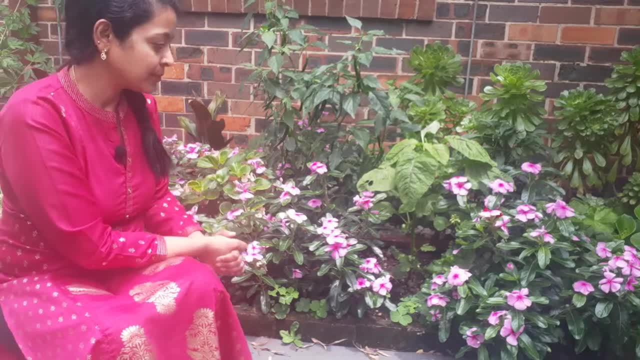 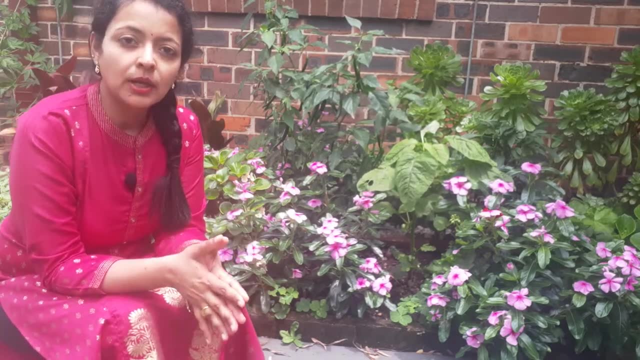 soil for a long time. So that is the reason why these leaves and these plants are healthy. but these problems do arise if you are growing it in the pot. So underwatering, overwatering- you have to take care of that thing if you are growing them in the pot. Now, apart from 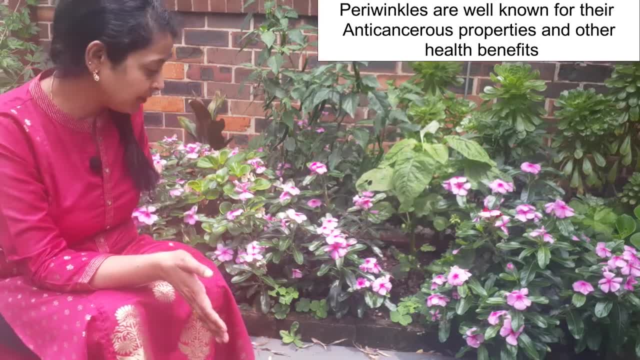 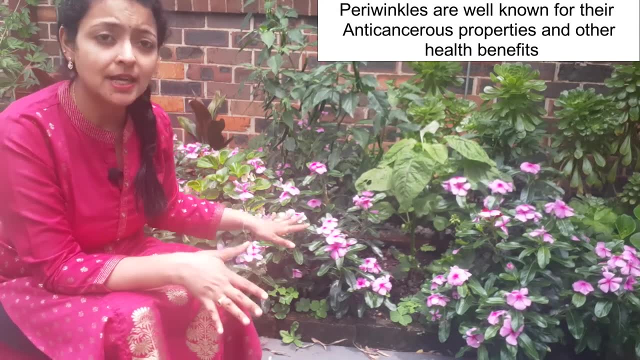 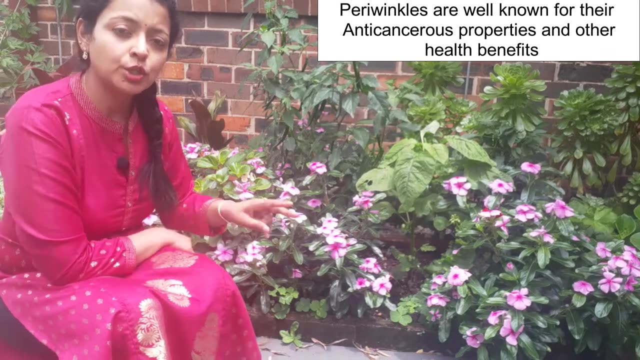 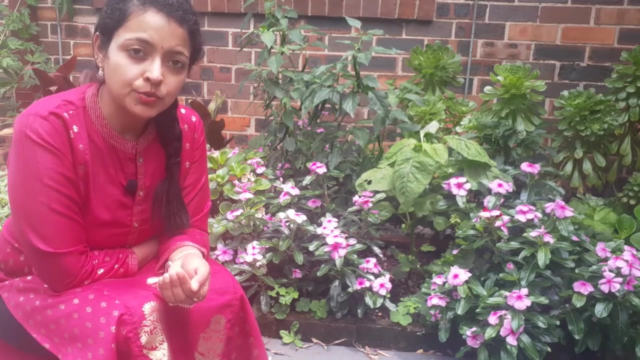 their beautiful display of these lovely flowers. these plants have got some benefits as well. So these benefits are that these plants are very well known- kind of famous- for their anti-cancerous properties. So these plants have got two substances in them, vincristine and vinblastine, and these chemical compounds are used, actually derived from the 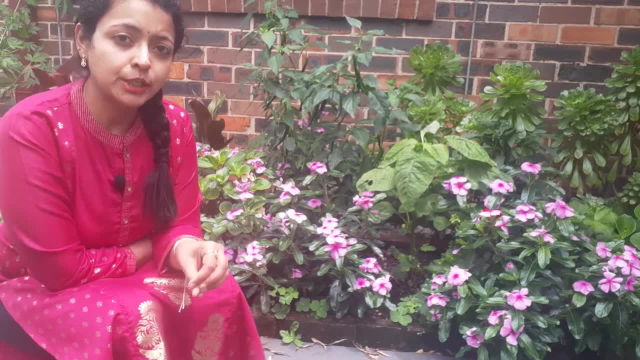 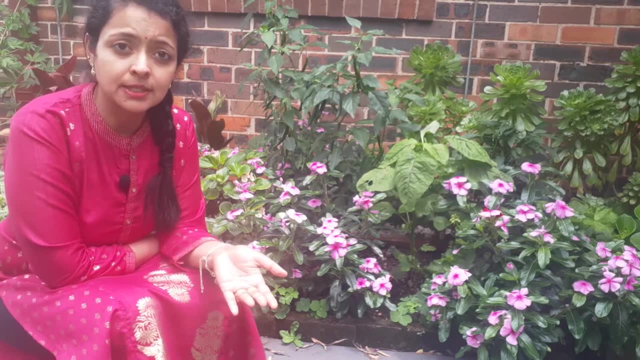 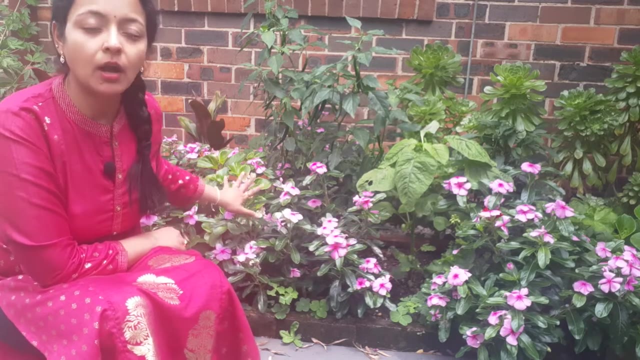 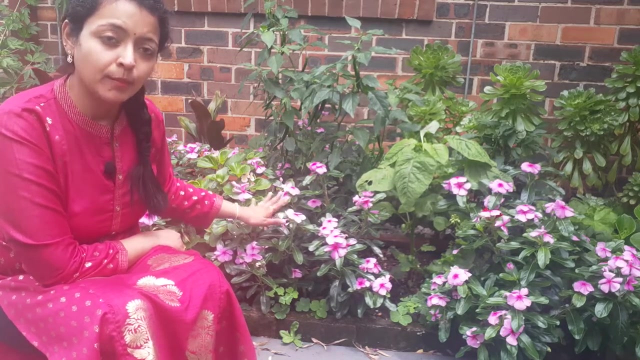 plant itself and they are used to treat leukemia, childhood cancers and lymphomas, Hodgkin's disease and many other sort of cancers. So those two drugs are anti-cancerous, which makes this plant a highly, highly toxic plant. So please keep this plant away from the reach of children and pets, because 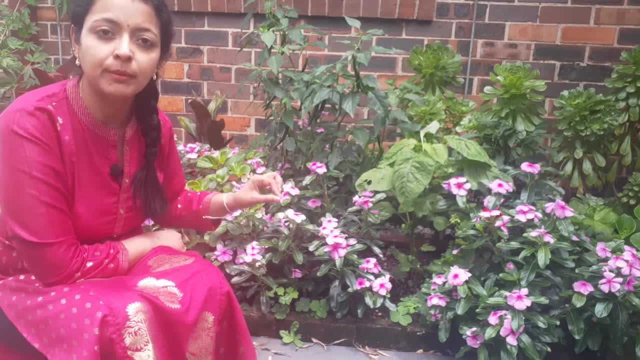 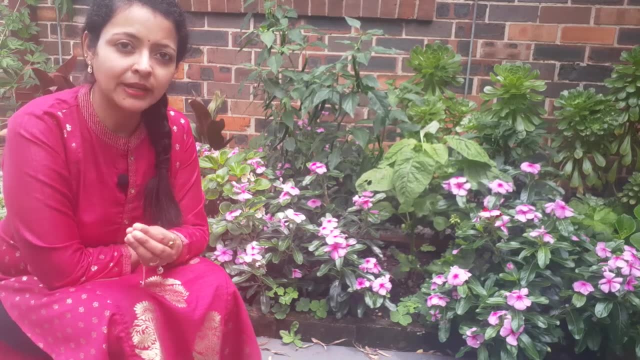 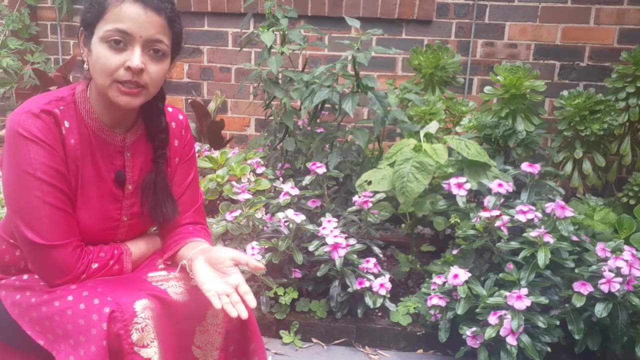 a little bit of ingestion of this plant can be very fatal for small children and pets. because of these two substances, because the anti-cancerous chemicals or anti-cancerous drugs. they are dangerous. Consuming those drugs can actually kill you. So do not eat these plants or do not. 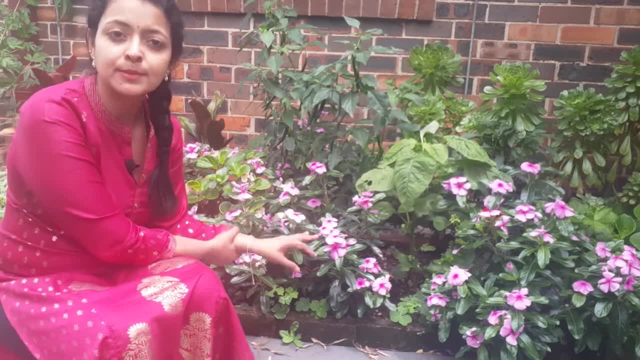 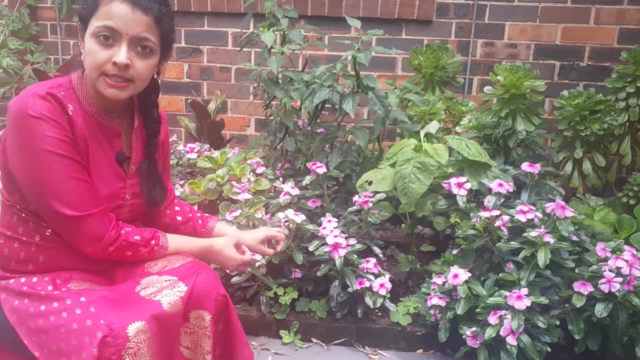 eat these plants. So do not eat these plants. or do not eat these plants, or do not eat these plants. If you want to use these plants, please consult your doctor before using them. Now. some people also say that having the tea made out of the leaves of these plants can actually help to cure. 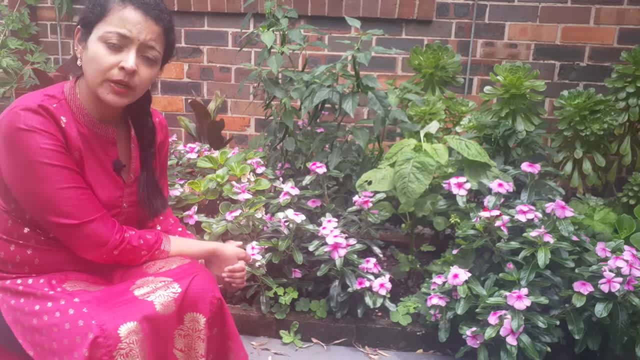 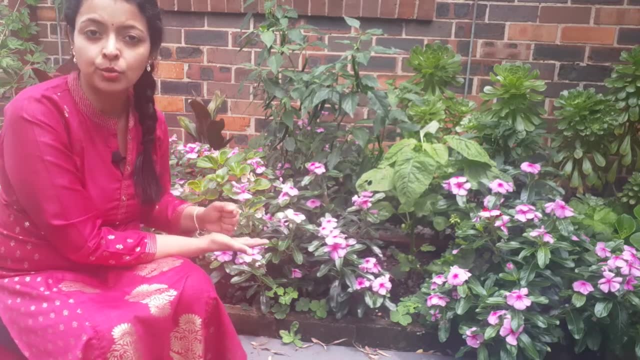 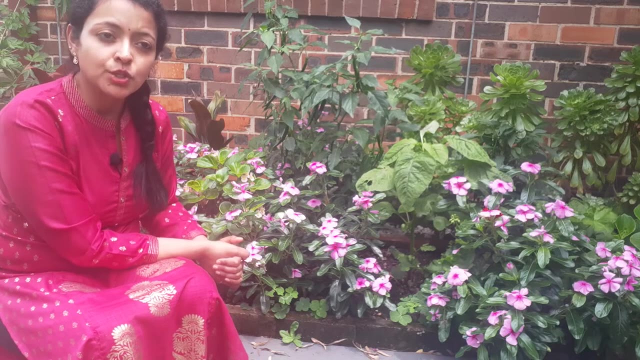 and prevent diabetes. It can detoxify the body, It can purify the blood and the flowers of these plants- if you crush them, make a paste and apply it on your skin- can actually help get rid of many skin infections and skin problems. So, honestly, I have never, ever, tried any of those things. If you, 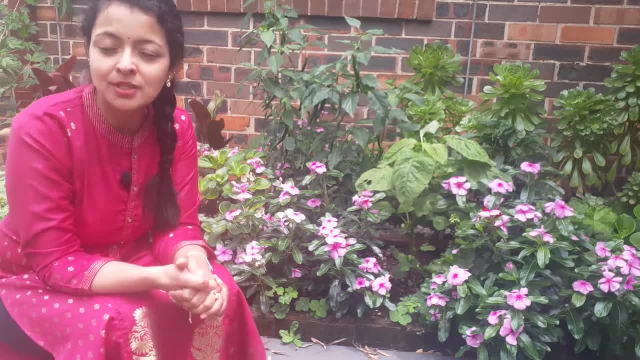 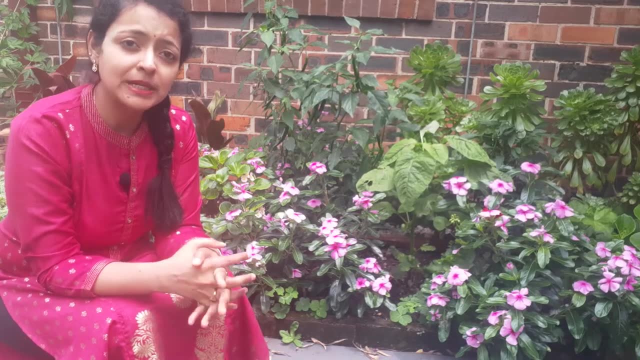 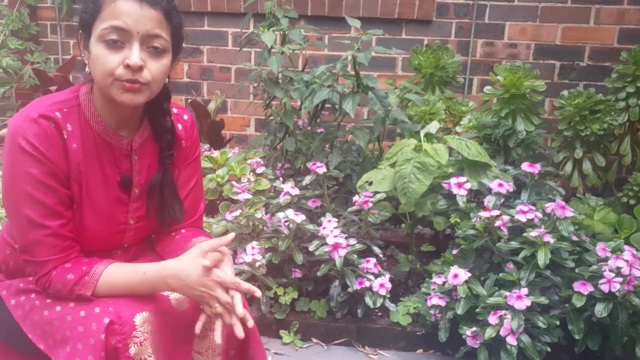 have tried any of them and it has worked for you, please share with us. do let us know by commenting down below. We will love to hear from you, but I have not tried any of those benefits that you can hear or you might read on different internet pages.